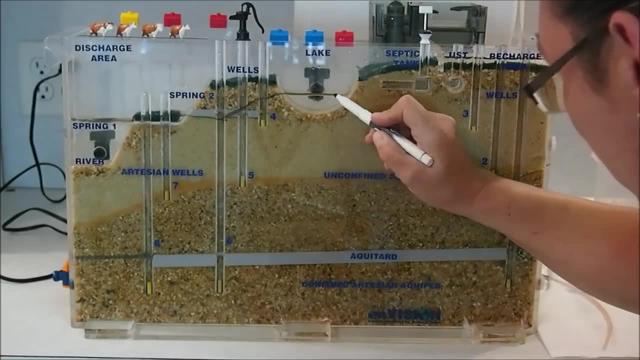 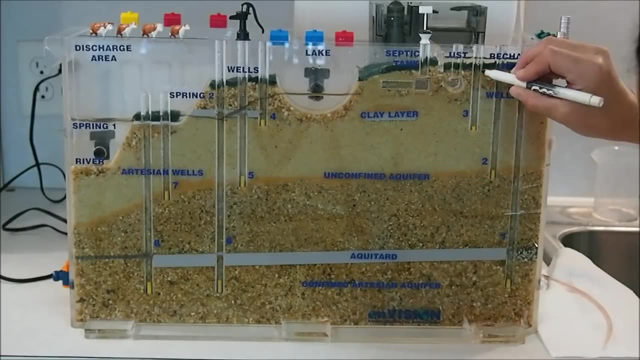 Water level's here there, And then I'll start with these wells and work backwards. So my water level is here in this one, So I'll just connect those lines Here in this one And here in this one. Okay, so that's our current water level. 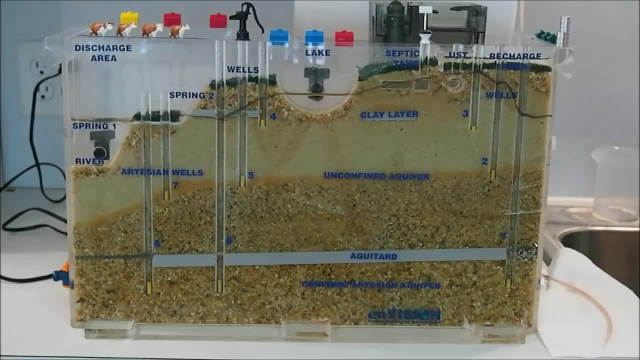 Now let's say we increase the flow, So we increase the recharge. Let's watch what happens to our water level then. Okay, so we can see our water level is rising. It's rising in our lake as well. now This one's moved up to here. 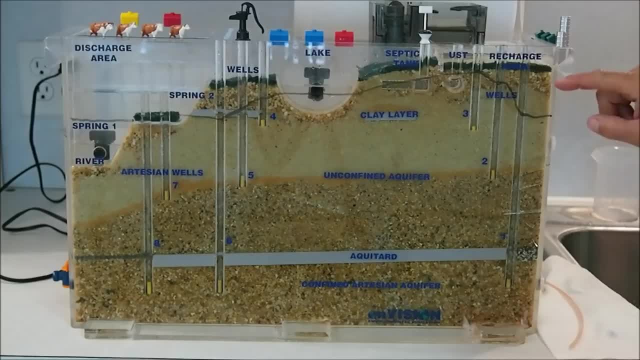 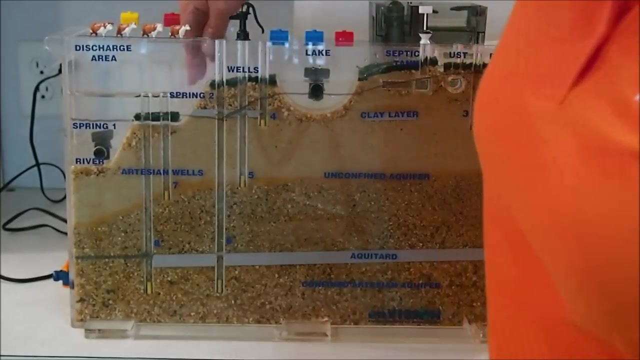 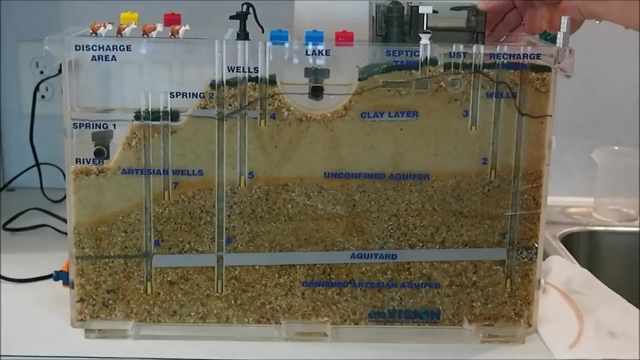 This one's up to here. This one's moved all the way up to there. This one's moved all the way up to there. So all of our water levels have now risen from increasing our recharge. I've increased the discharge And you see they're falling rapidly just by increasing the discharge. 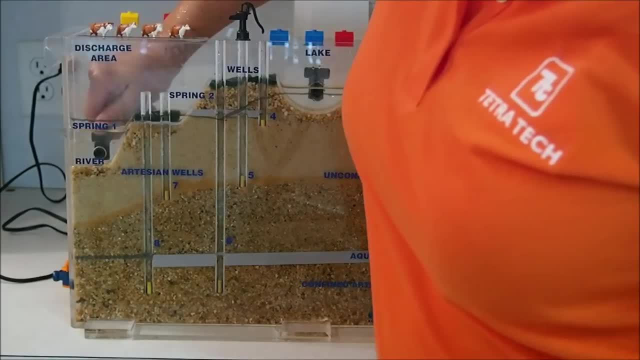 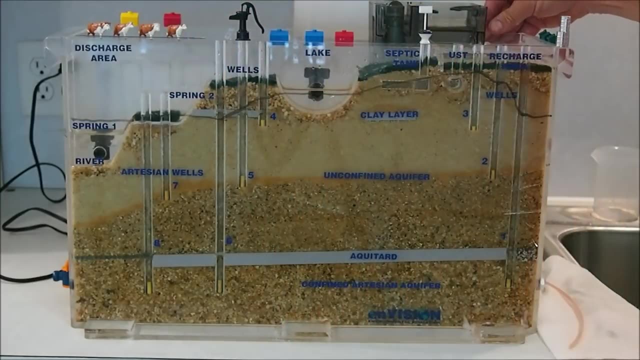 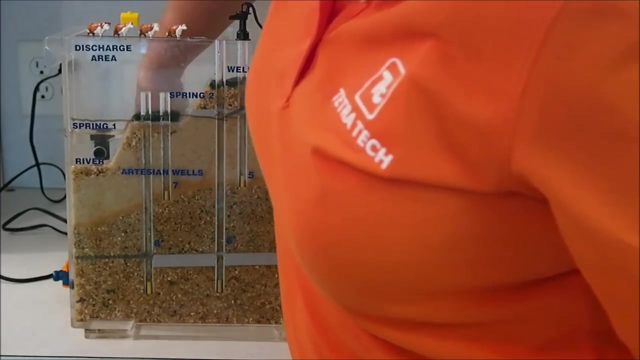 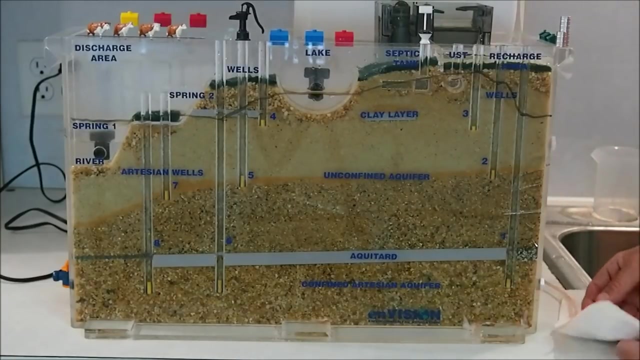 So let's go ahead and get this stabilized again. I keep knocking my houses off. Okay, I think we're pretty close to having our water level back where it was before. So how do you think you can measure the water level in the real world? 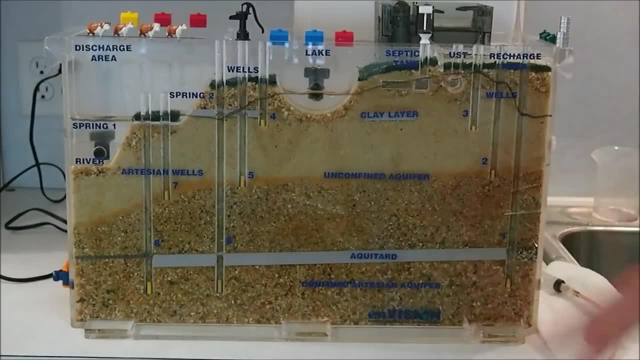 Obviously, you can't cut a cross-section of the earth and see it like this, But what are some things you think you could do? I mean, we're capable of drilling wells, right, And we're also capable of measuring the water level in wells. 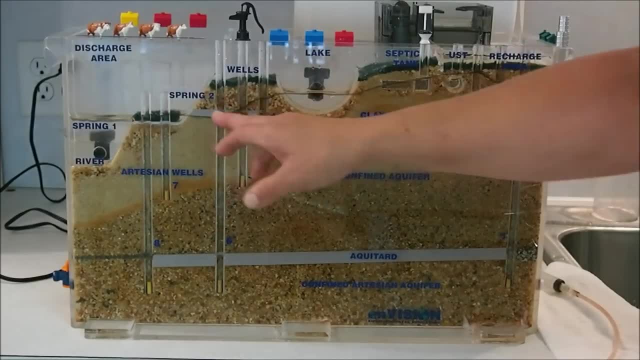 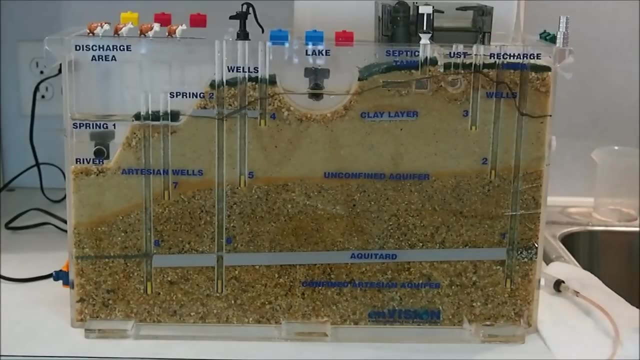 So perhaps you could measure the water level in all the different wells, Drill a variety of wells, measure the water level and that would give you a good indication of what your water level is. And actually that's what hydrogeologists can do and do do. 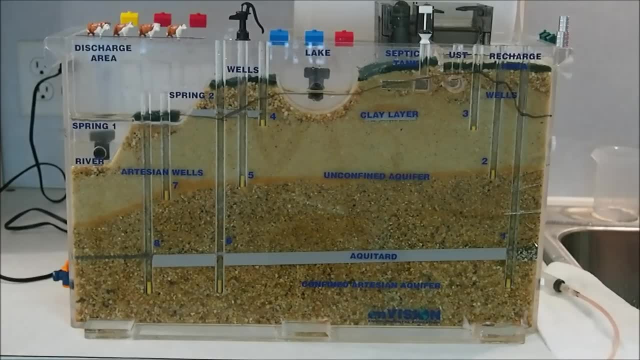 So why do you think we had that change when I increased the recharge? Why do you think we had the change in the water level? Think about it for a minute. The water table itself is really based on your recharge and your discharge right. 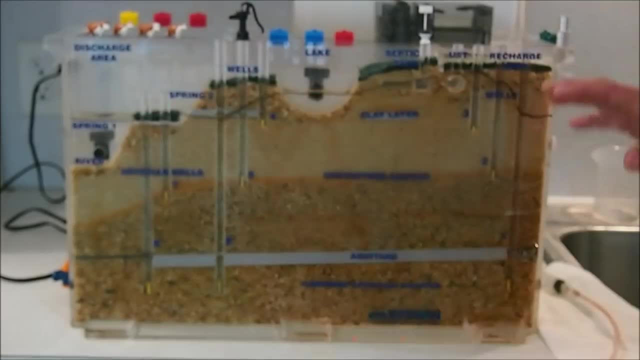 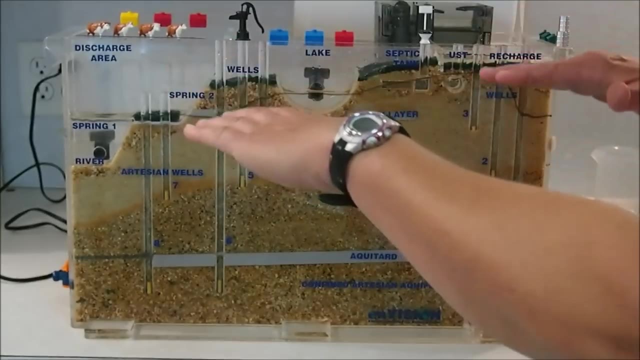 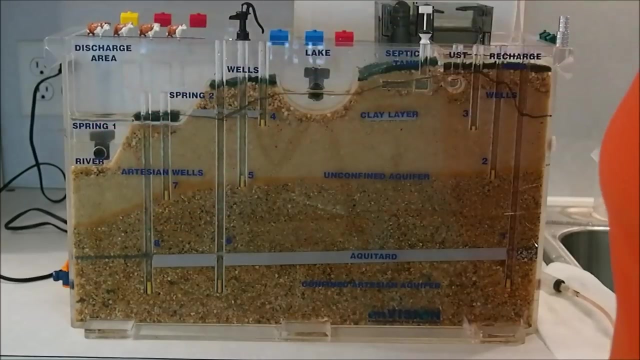 So there's a pressure differential. that's happening there. You've got water coming in, it's pushing water through and then water is leaving the system And when it balances you've got about the same amount coming in as going out. You can see I've even got a little more going. 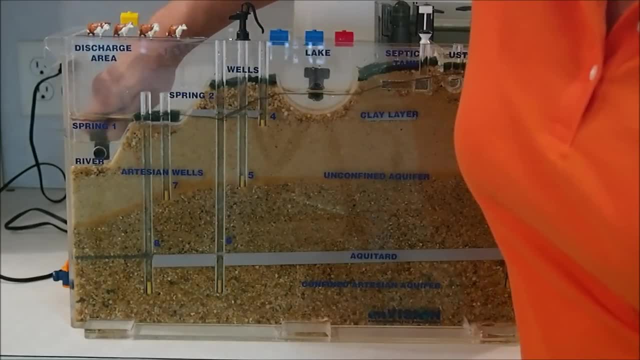 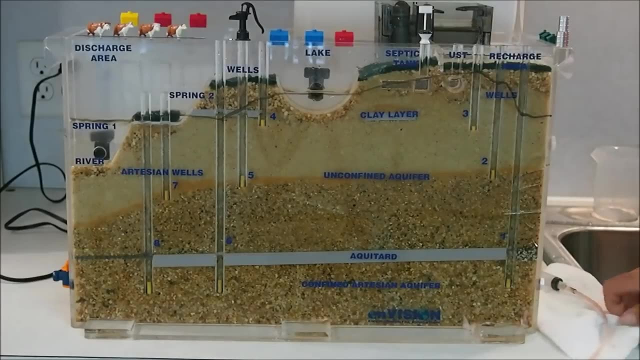 In than out now, because my water level is still rising slightly. Okay, so what we're going to do is we're going to introduce some dye into some wells. We're going to calculate the velocity of flow of our system, That is, the amount of water coming in and flowing through our system. 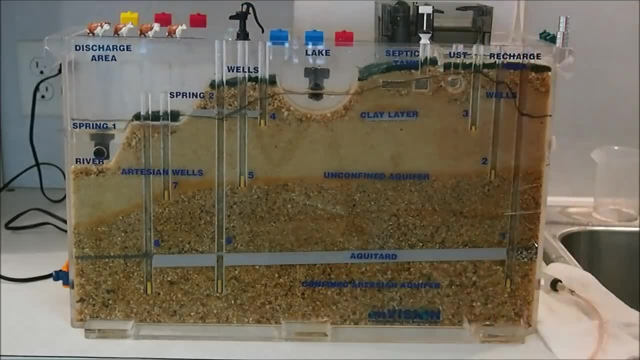 And velocity is calculated by distance over time. so distance divided by time. But first what we're going to do is we're going to pull some sand or some water out of the fine aquifer. So this is our fine aquifer here, this fine layer of sand, and I'm going to put a syringe in here. 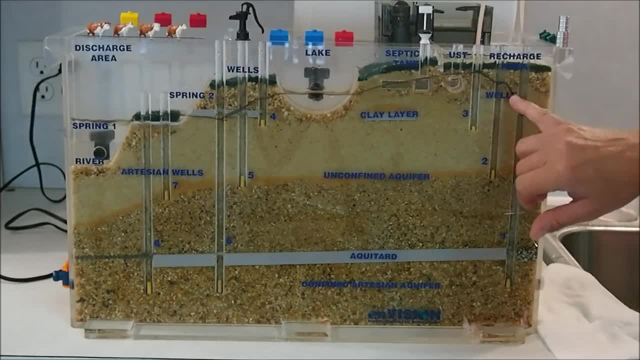 and draw some water. Okay, So we're going to draw some water out and then we're going to watch what happens to this water level. So I'm pulling water out of this and my water level now in this one is down here. 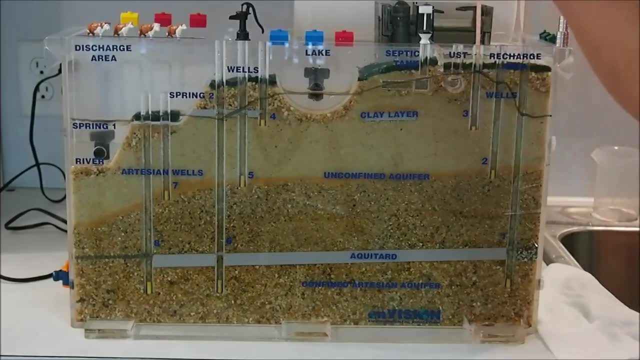 So what happened there? Let's do it again here and see I'm drawing water from this well, And now this well is down here, starting to rebound a little bit, but it dropped really rapidly when I pulled water out. There's a name for that. 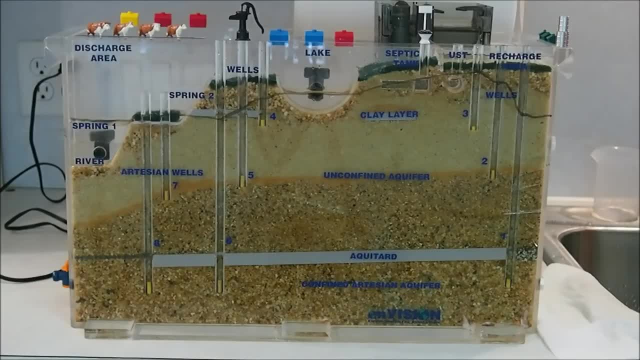 Hopefully you've gone through that in lecture. So let's see what happens when I go into the coarse sand aquifer. I think this one takes me into there, So I'll go ahead and put this one in here and I'll draw water up. 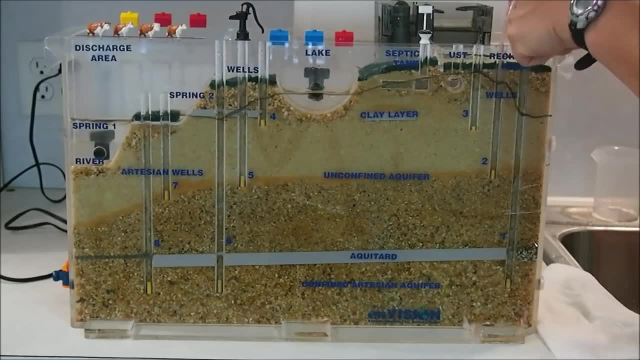 Again, our water level on this one- oh, my contaminant barrels fell. Okay, our water level on this one is actually up here now, so we must have a little more recharge going in than what we had originally. Let me draw from here. 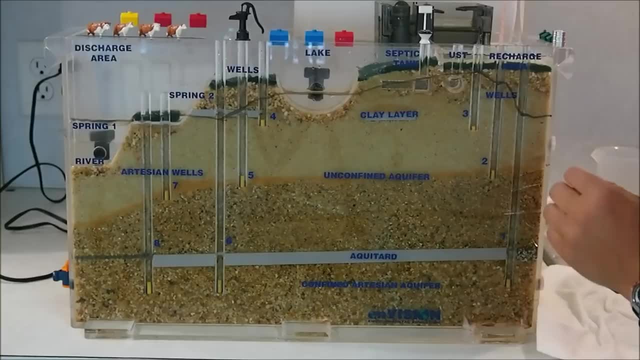 Oops, And the water level just dropped a little bit. Okay, There we go, Oops, And the water level dropped, but it's rebounding right back. Let's try it again. I can show you where the water table ends up. 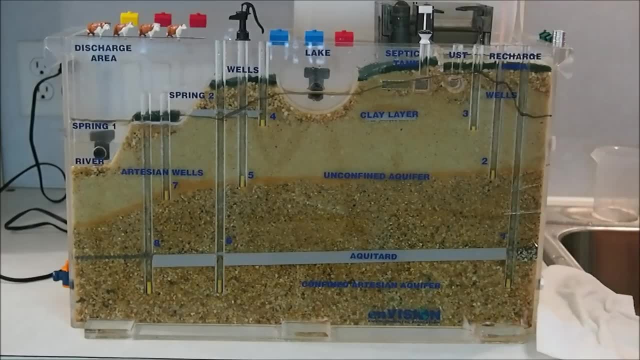 Yep, it went right down and now it's coming right back up. All right, so let's go ahead and do velocity calculations And we're going to start out. Okay, So we're going to start out with the fine sand aquifer. 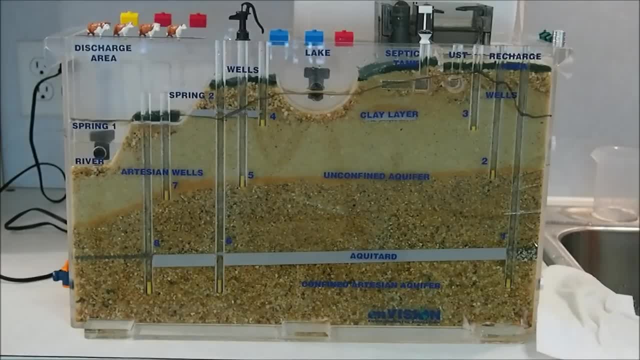 And the fine sand aquifer. Now you had a timer of some sort before, whether it's your watch or your iPhone, again to do the minutes and seconds. So I'm going to do the measuring part. I'm going to introduce the dye and do the measuring part and you're going to do the 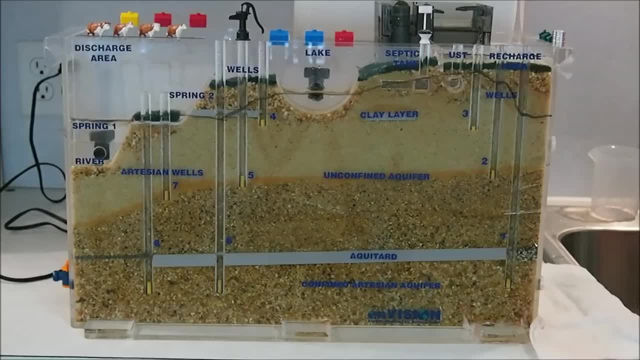 timing part. So let me get a little bit of dye in my syringe. We'll call this a contaminant. Okay, So I've got my barrels of contaminated barrels of toxic red waste and I'm going to introduce these into a well. 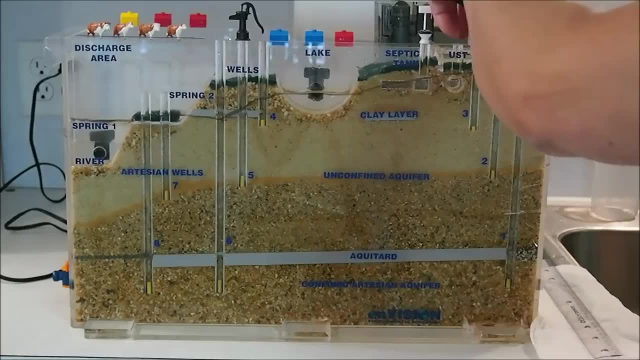 All right, We're going to do this in the fine aquifer. so that's right here. well, number three. And again, we're going to do this in the fine aquifer. so that's right here. well, number three, Okay. 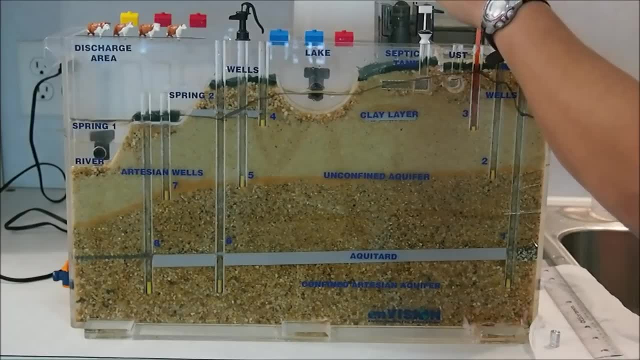 So we're going to do this in the fine aquifer, so that's right here. well, number three, And again, when I tell you to go, you start your timer, and when I tell you to stop, you'll stop it. 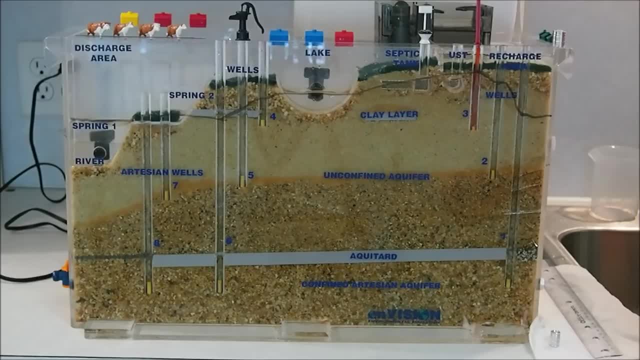 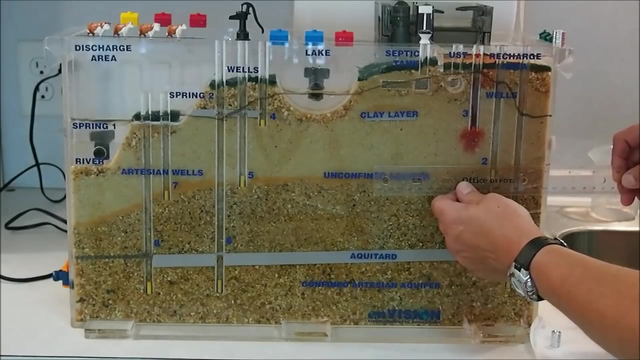 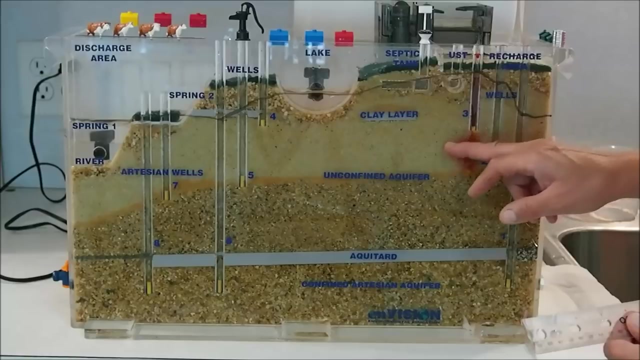 All right, Ready, Set, Go, Okay, And you can see, this is what they would call a plume if it was a contaminant. So our dye has been introduced into the sand, the unconfined aquifer, the fine sand aquifer. 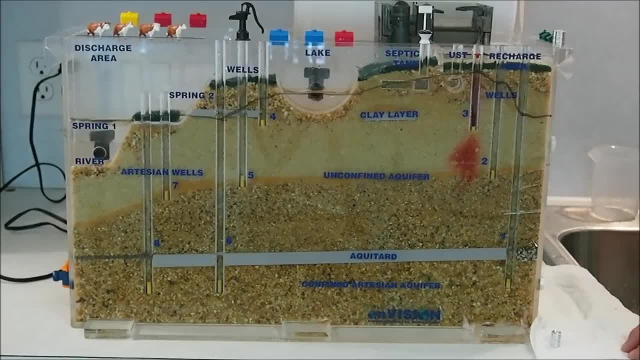 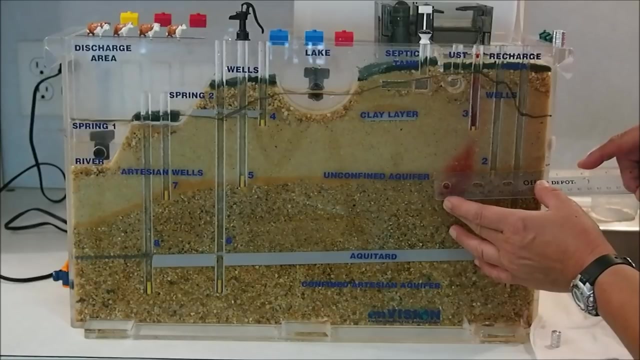 And if you're watching it, think about which way it's going. Okay, Okay, It is moving down a little, but primarily it seems to be moving with the flow of the water. Okay, It is moving down a little, but primarily it seems to be moving with the flow of the. 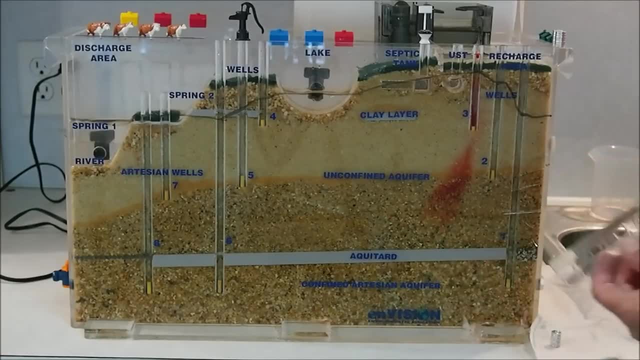 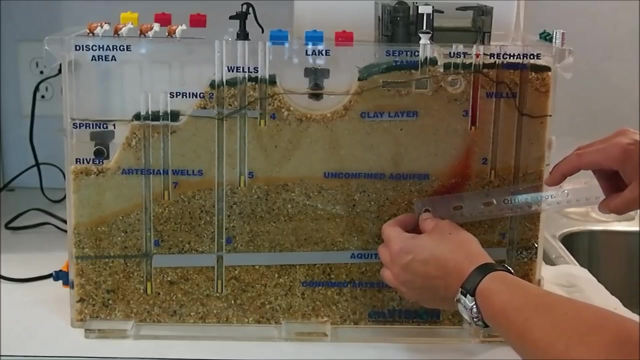 water. Okay, It is moving down a little, but primarily it seems to be moving with the flow of the water. We've seen the movement. We've moved down probably about three inches over about two. We're going to go just with the over for velocity because we're following the path of the water. 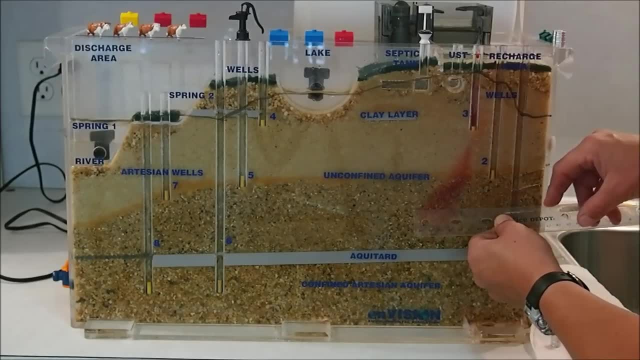 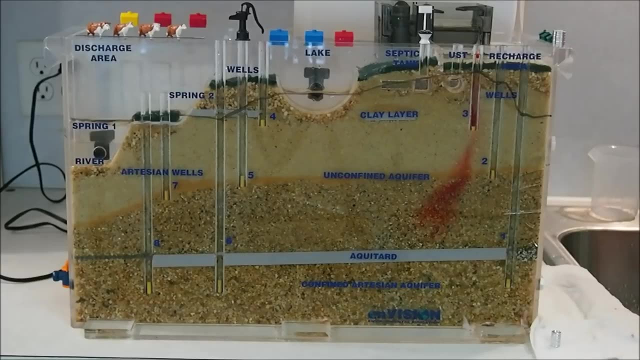 so I'd say we're at about two inches now, So let's go ahead and stop the timer. Okay, Okay, We've moved around the top. Okay, distance over time, so that two inches over how many ever seconds that your watch was at, and that's going to tell you how fast the water is flowing now. 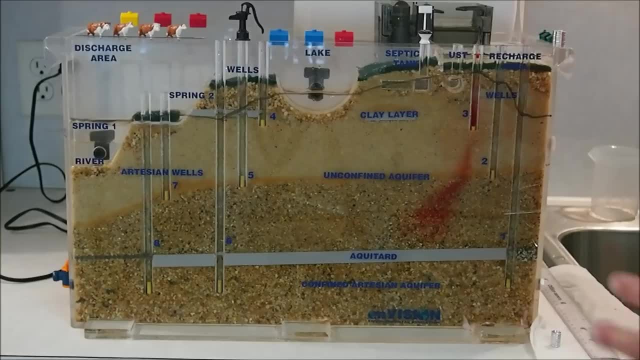 again. think about it for a minute. if you've got a recharge coming in, this water is coming in here and discharge is going out, so it's going out there. so which direction is your water flowing? is it flowing from recharge to discharge or from discharge to recharge? that might be a question that you need to think about. 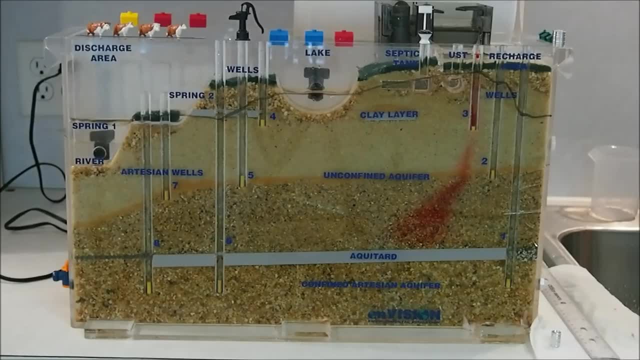 all right, so go ahead and calculate your velocity for that one and think about what happens to the contaminant that I put in there. so you think I got darker. okay, so I'm going to go ahead and calculate the velocity for that one and think about what happens to the contaminant that I put in there. so you 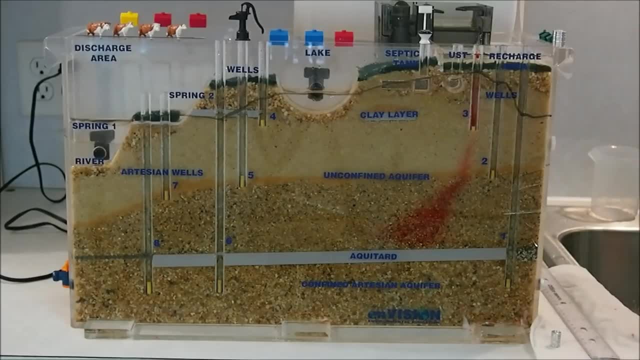 or did it change color at all? did anything happen? it started out kind of a small bubble there and now it's pretty big and spread out. but what happened with it? did it did so? think about that for a moment. let's see what happens when I try to withdraw a little bit of it. 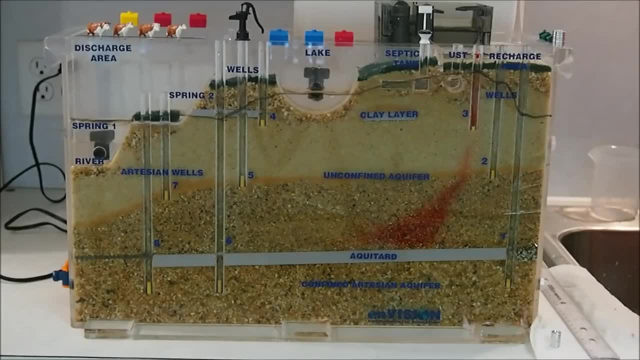 I'm going to rinse some of this out of here so that I don't have to put that in to do some more. I missed most of it, right? but you can see up here the sand is almost clear, right, and then it gets pink again. I missed most of it, right, but you can see up here the sand is almost clear, right, and then it gets pink again. 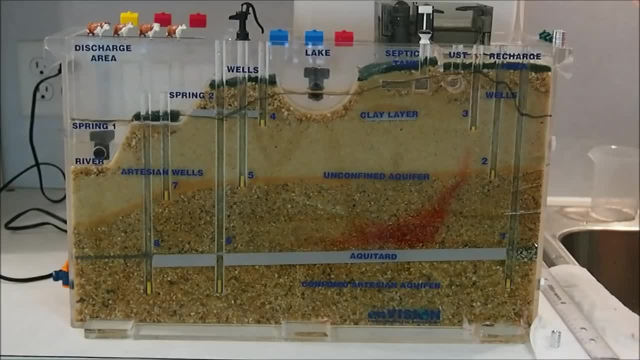 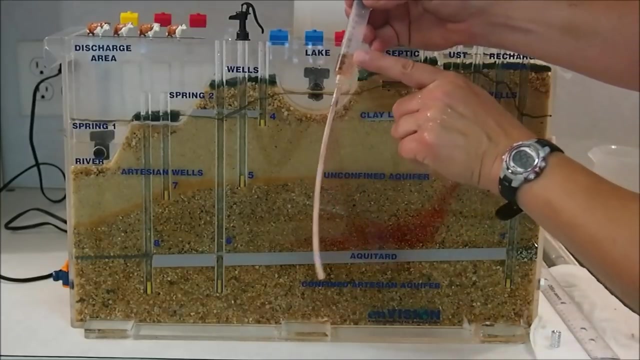 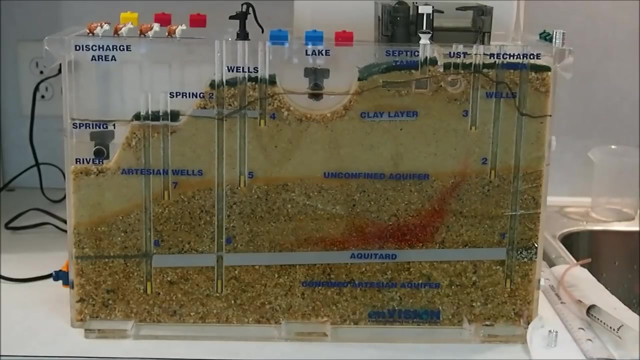 water I'm just charging was pink. see the water in the tubes. the tubes died pink anyway, but you can see in the syringe here the waters pink. all right, notice what happens to when it hits the aquitard. okay, so let's see what happens when we try this out in the 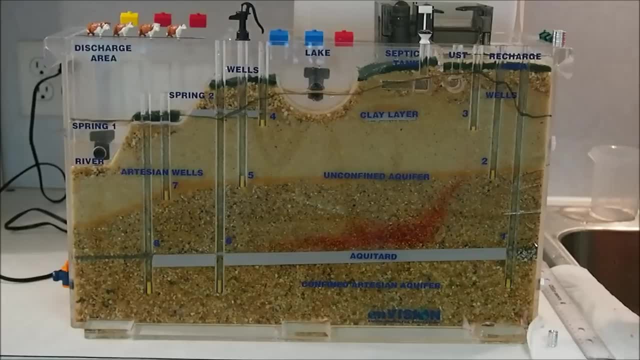 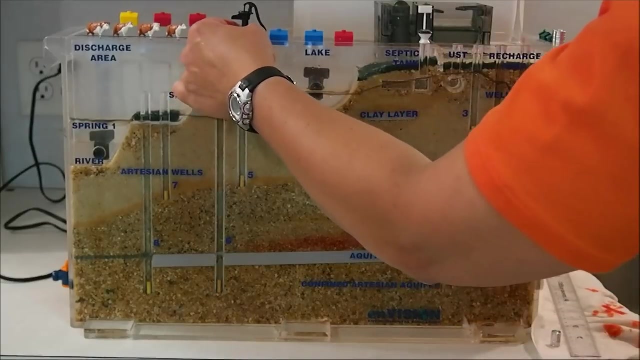 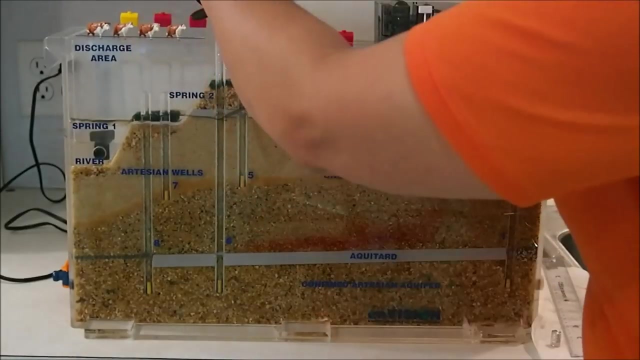 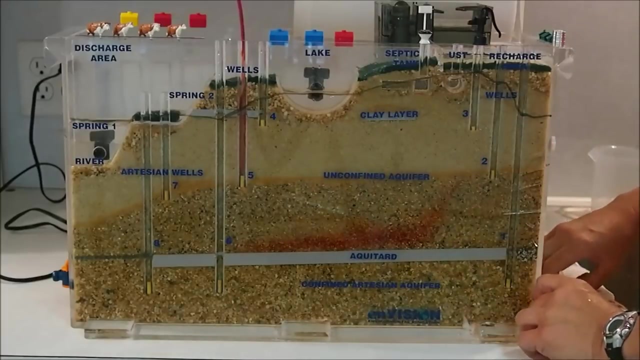 coarser, coarser sand. think I'm going to have red fingers for a couple days, alright, so let's try it out over here a little. well. well, to where the other wells are, All right. so reset your timer to zero. ready set go. 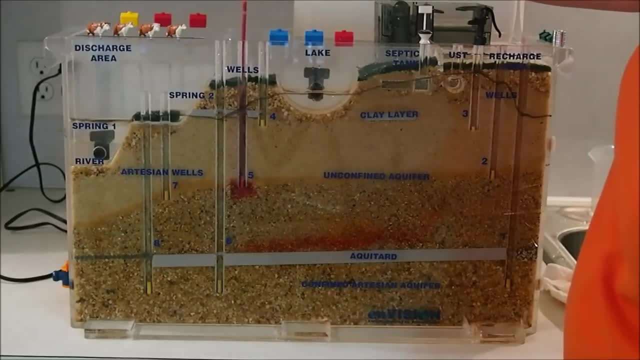 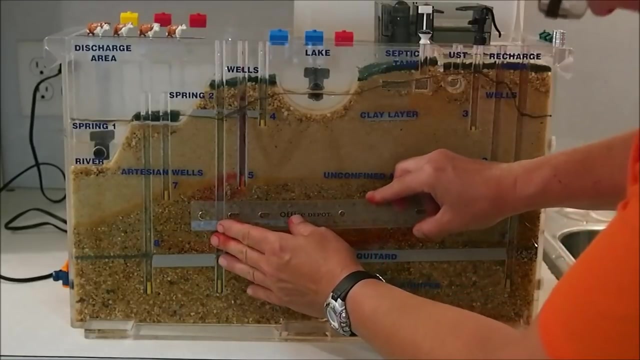 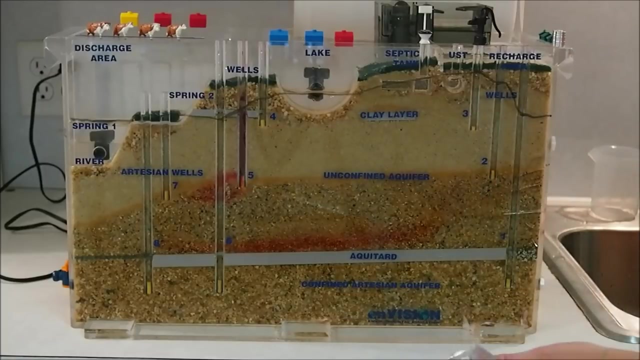 Again. I start out with my little plume here. You can see it's already over here. All right, stop. I'm at two inches already, which is what we had on the first one, right, So check out the time for that. 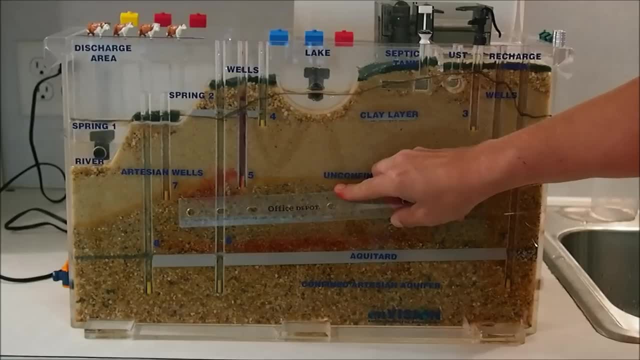 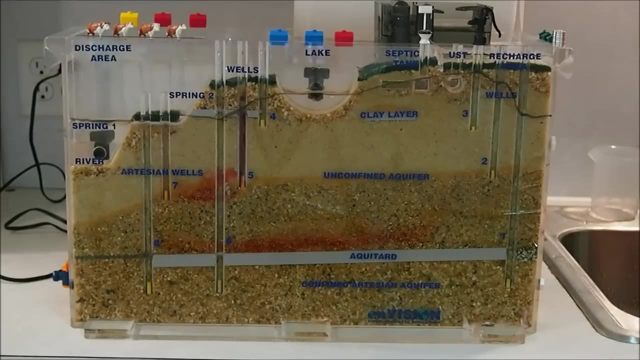 That was: yeah, it's already at two and a half. It's moving pretty rapidly right across this coarse grass, Gravel mix, sand, gravel mix, Okay. so again think about which direction that dye is flowing. Is it flowing from recharge to discharge or discharge to recharge? 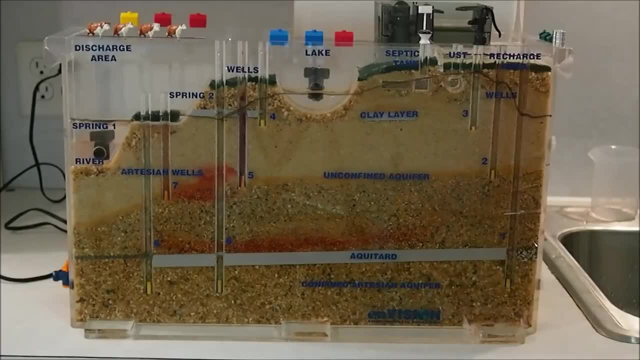 And what's happening to the dye. You know it kind of started out in that clump here. It was really dark. I'll clean the tube out a little bit here. take some of the dye off, Get the syringe nice and clear again. 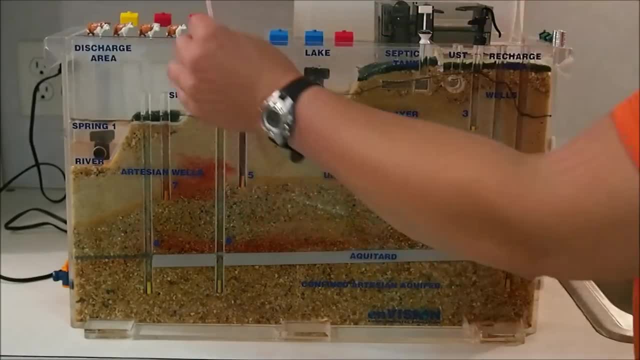 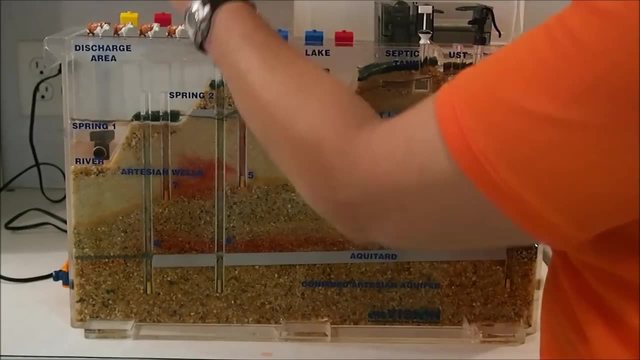 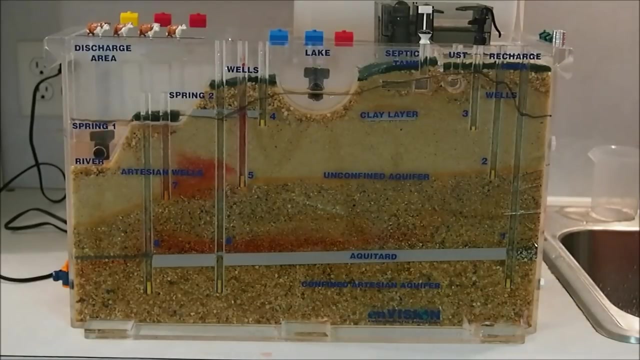 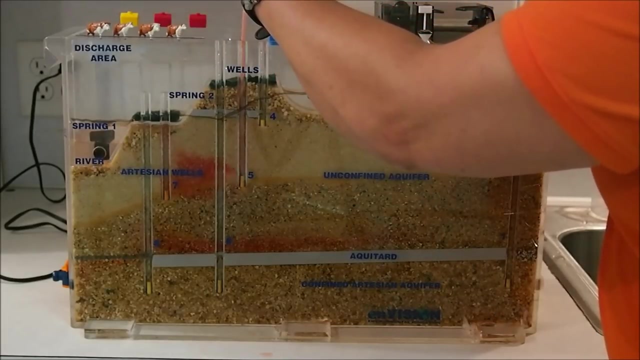 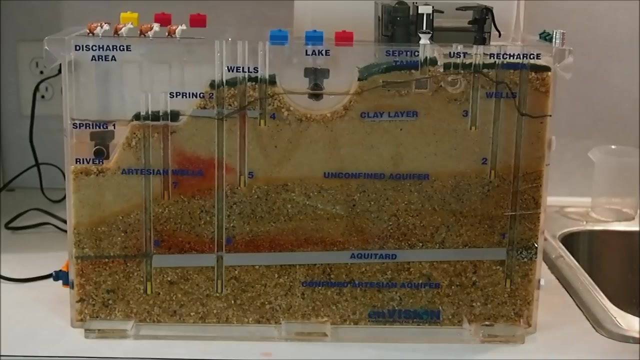 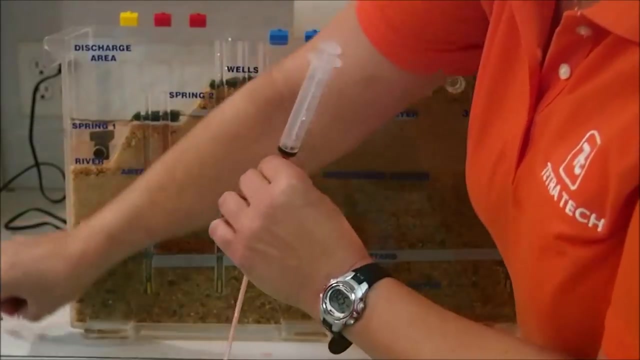 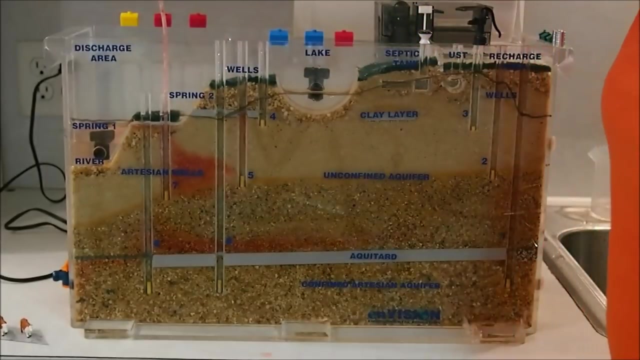 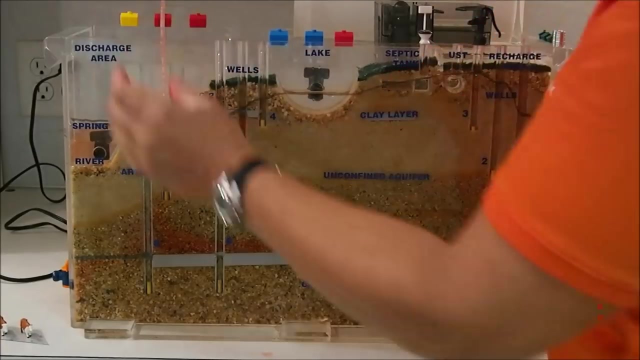 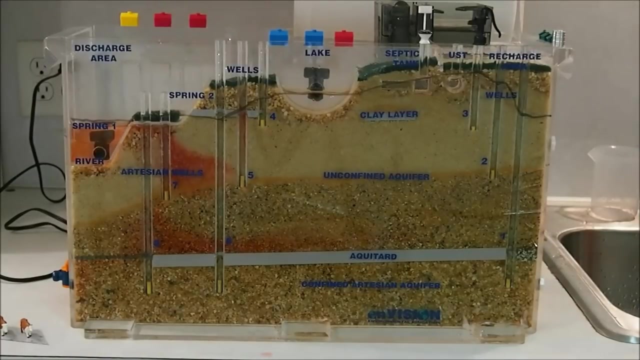 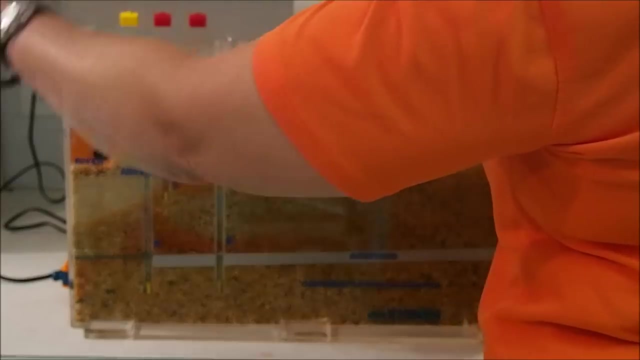 See, the syringe is very clear. So what's happening when I do that? Let's see if I move my little cows here. Well, look at that. well, Alright, so go ahead and zero your timers again, And we're going to try one more. 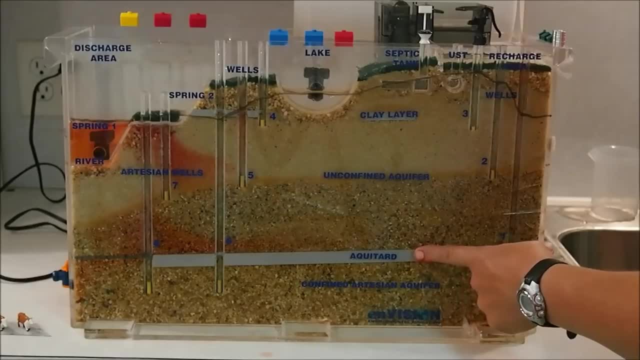 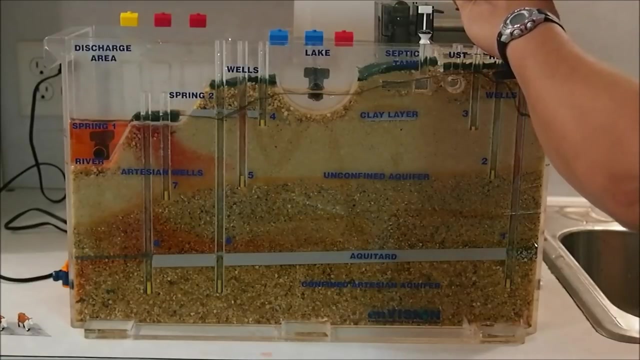 Alright, so I'm going to come back over here, I'm going to go beneath this one And I'm going to go beneath the aqua turd into this coarse gravel mix. Alright, so are you ready? Start your timer Again. you can see, we've got a nice dark plume right there. 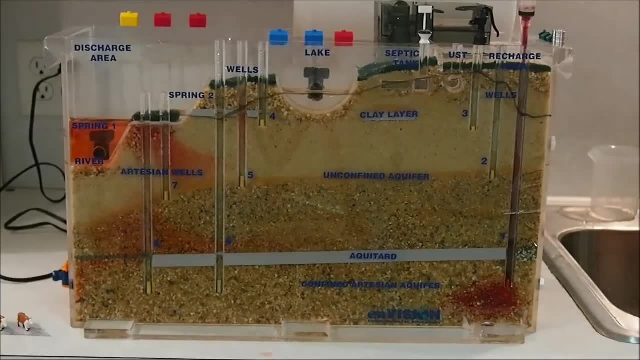 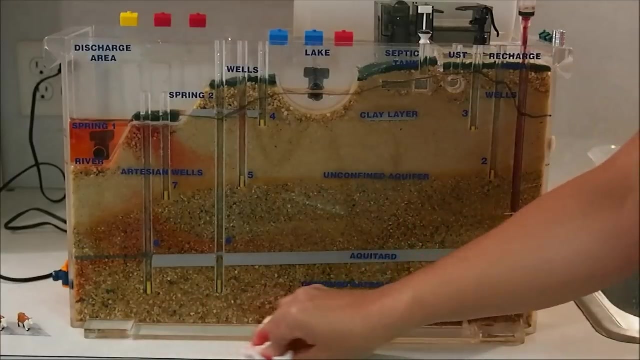 The contamination. We are already at 2 inches, So we're at 3 inches. Start your timer Again. calculate the velocity Distance over time. You just divide it out And that will give you inches per second. Look at that. 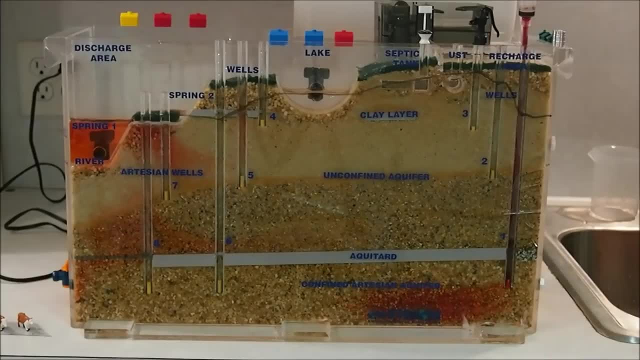 Look how fast that's moving. Again, I pull it back up. Oh no, It knocked over my. well, Let's see what happens right around the bottom of this. Let's see what happens when I'm pulling it out. Okay.